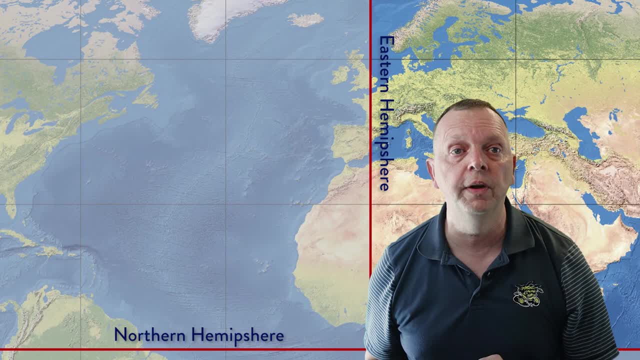 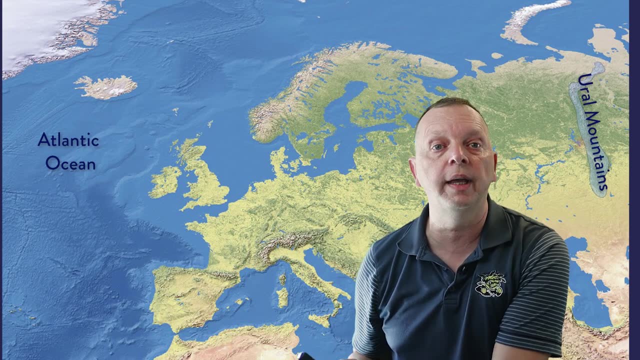 We find Europe, most of Europe, in the Northeastern Hemispheres and we find that it stretches between the Atlantic Ocean in the west all the way to the Euro Mountains in Russia in the east, and then from the north we go from the Arctic Ocean all the way down to the Mediterranean Sea in the south. 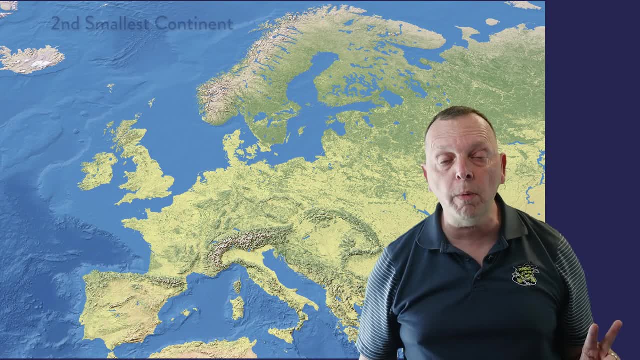 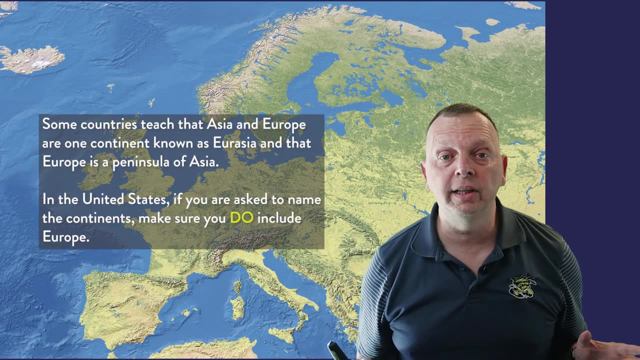 Now, Europe is not a very large continent. In fact, it is the second smallest continent in the world, right after that of Australia. but technically Europe actually isn't a continent at all. In fact, we actually see that Europe is a peninsula of peninsulas. 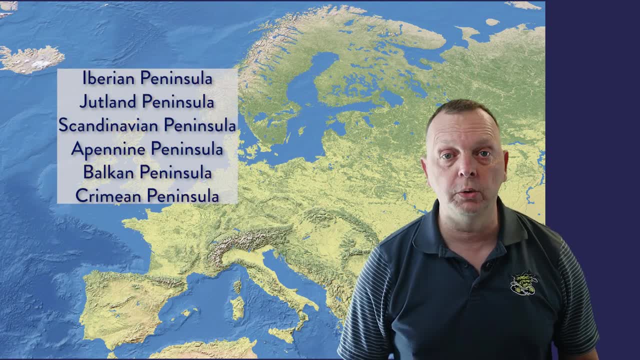 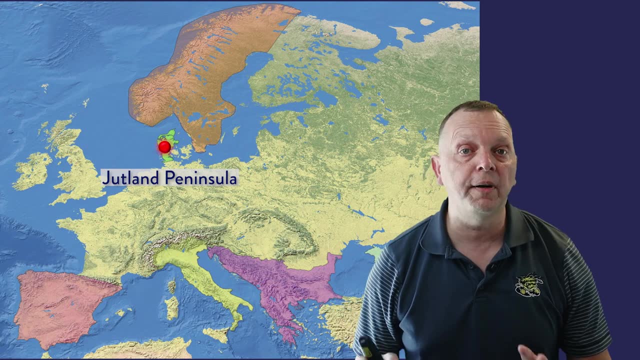 There are six major peninsulas that define many of the countries of Europe. There is the Iberian Peninsula. It is made up of Spain and Portugal. In the north is the Jutland Peninsula, where we find Denmark. Then there is the Scandinavian Peninsula, which is the landmass which we find Norway and Sweden. 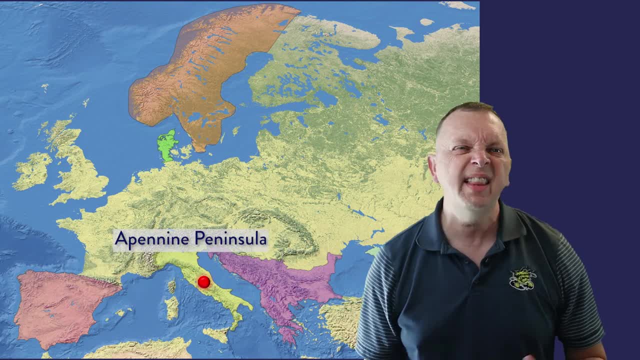 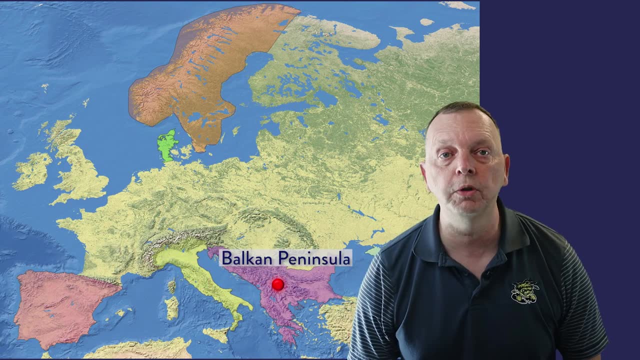 Now, if we go down to the south, we find the Apennine Peninsula, That's the northern part of Europe, That's the one that looks like a boot in the Mediterranean. This is the peninsula that makes up Italy. Then we find the Balkan Peninsula, which includes Greece. 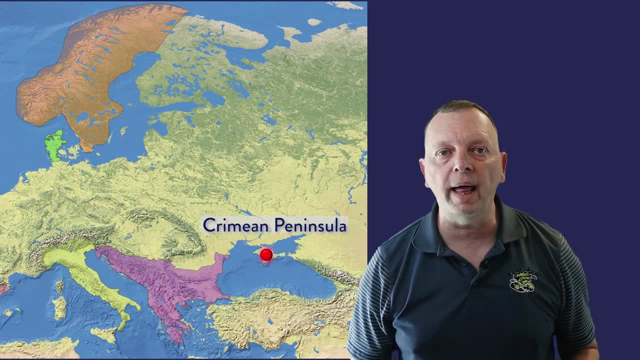 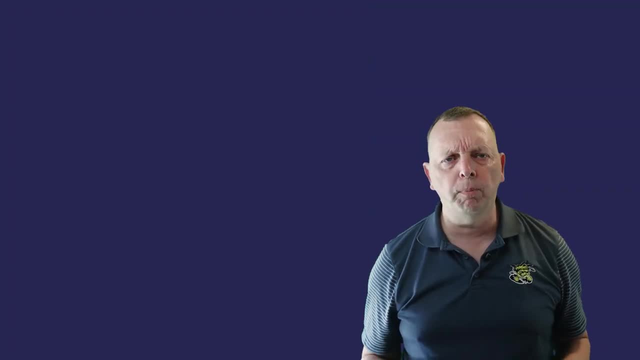 And then there is the Crimean Peninsula that juts out into the Black Sea. It was once part of Ukraine until a few years ago, when Russia invaded and took it over Now. peninsulas are surely important to Europe, especially since we find that itself is a peninsula. 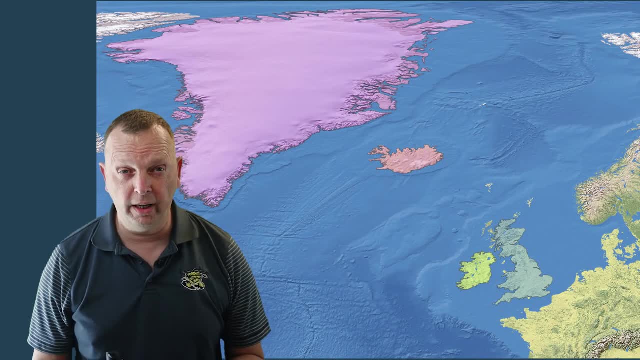 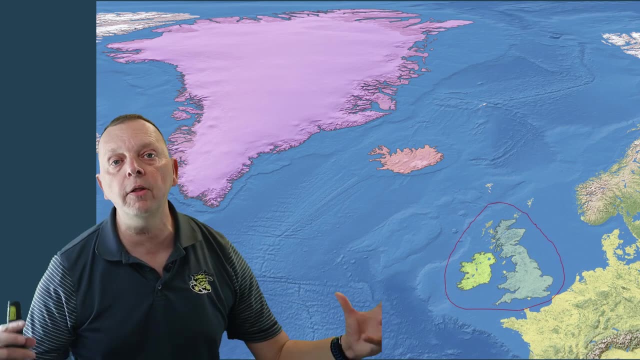 but so are islands. We see several important islands in the northeast, just across the English Channel, from France's Great Britain to its west, you will find the island of Ireland, And together these all make up what is known as the British Isles. 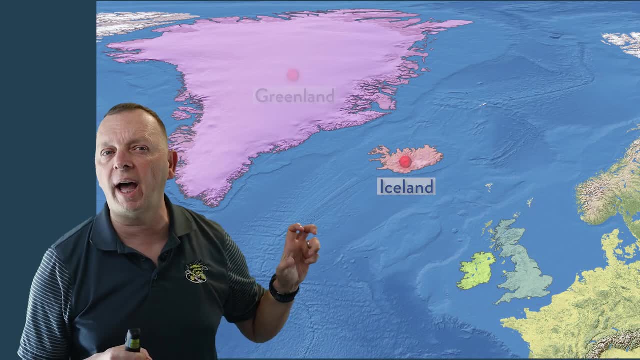 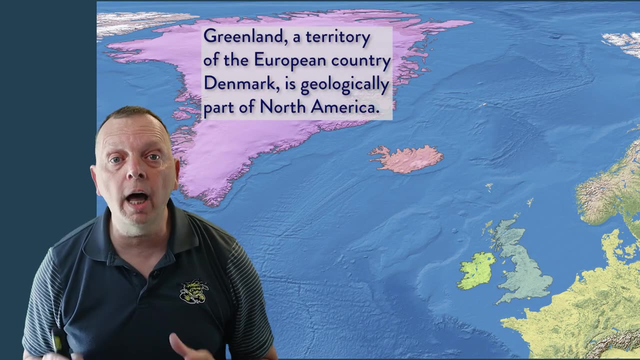 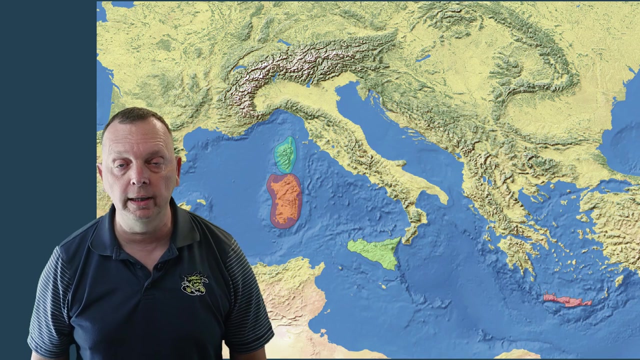 Now, to the northwest of Ireland is Iceland and to the west is Greenland. Of course we might be cheating a little bit here, because although Greenland belongs to Denmark technically, geologically Greenland is actually part of the North American continent. Now, if we go down in the south, in the Mediterranean, there are several islands of note. 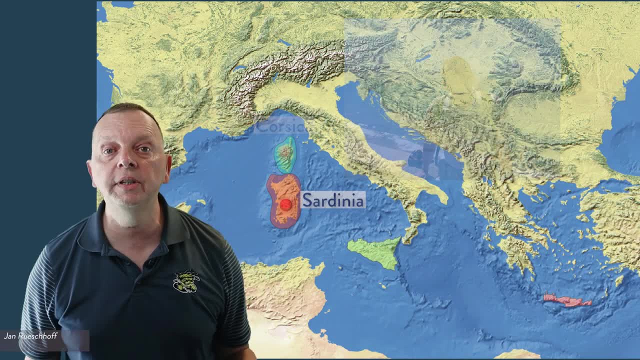 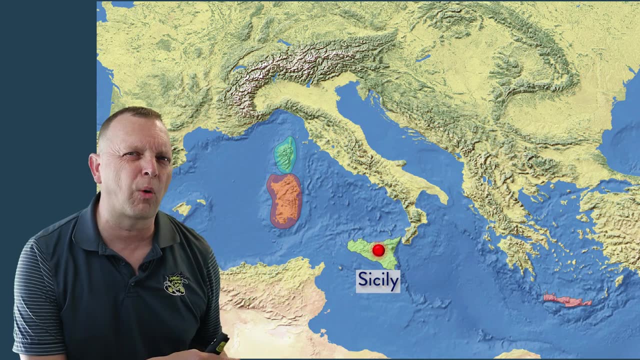 Corsica, where I am in this picture, is part of France, and to the south is Sardinia, which is a territory of Italy. Also in the territory of Italy is Sicily, and this, essentially, is kind of like the rock through the boot of the Apennine Peninsula: looks like it's kicking. 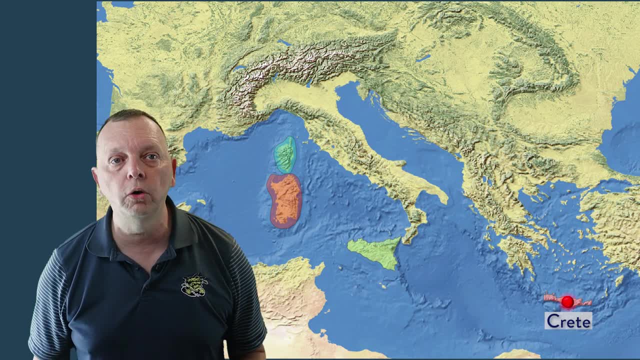 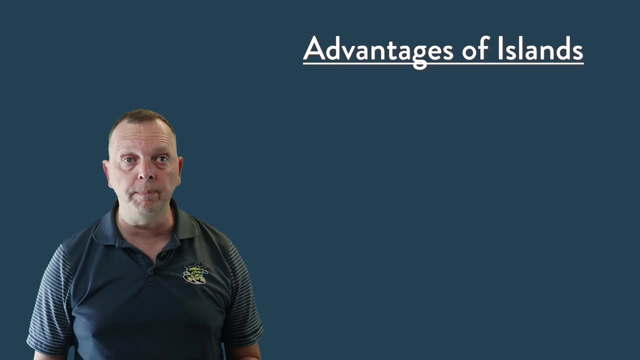 And further to the east, we find Crete, which is the second and the largest populated island of Greece. Now, islands do have advantages, especially if you are an island country such as Great Britain. First, since islands are normally surrounded by water, they have easy access to the ocean. 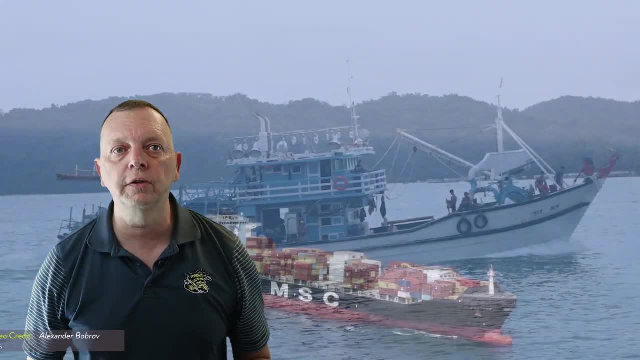 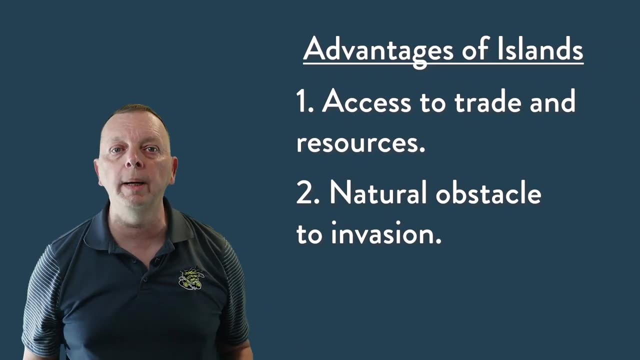 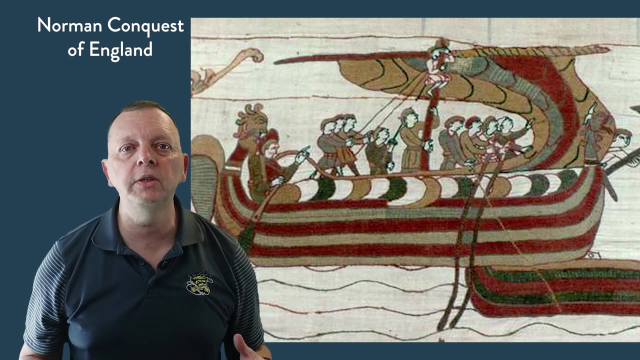 This allows for increased maritime trade and other resources such as fishing. Second islands are also more difficult to invade because of the difficulty of crossing the ocean with an army. An example again is Great Britain. Now. while they were invaded a couple of times in their history, their island status is what has protected them from being invaded by Hitler during World War II. 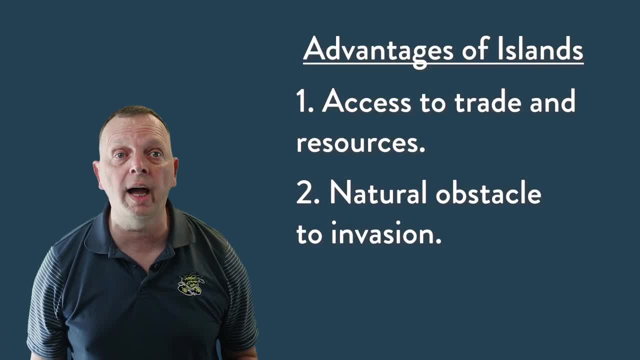 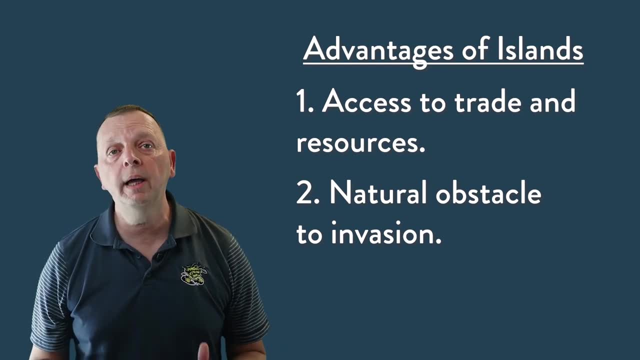 In the early days of sea travel, getting from one point to another took actually a long time. Ships several hundred years ago were really nothing more than just big boats, and they couldn't carry a lot of supplies. Because of this, islands became stepping stones for a year. 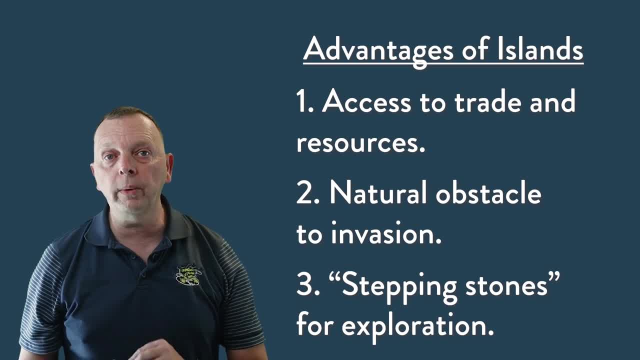 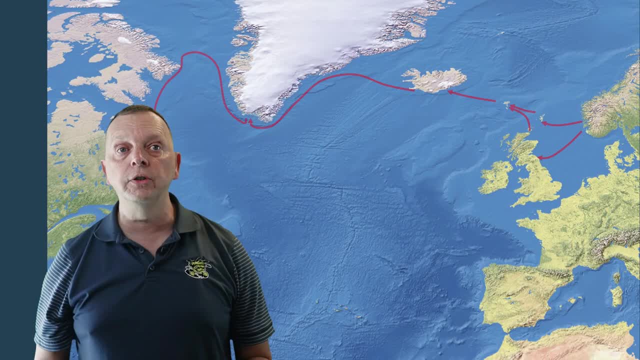 However, in the early days of sea travel they were able to carry a lot of supplies. Take the Vikings. These were the people of Denmark, Norway and Sweden. They used the British Isles, Iceland and Greenland to get to Canada and North America around the year 1000. 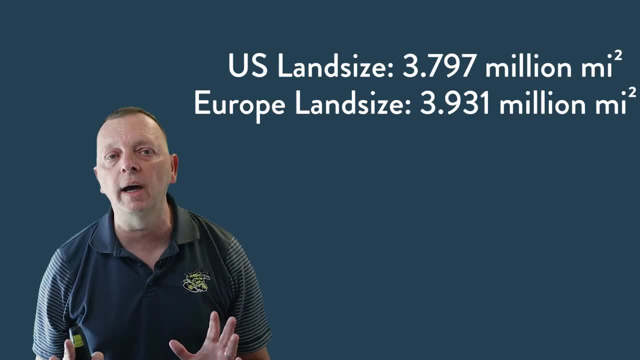 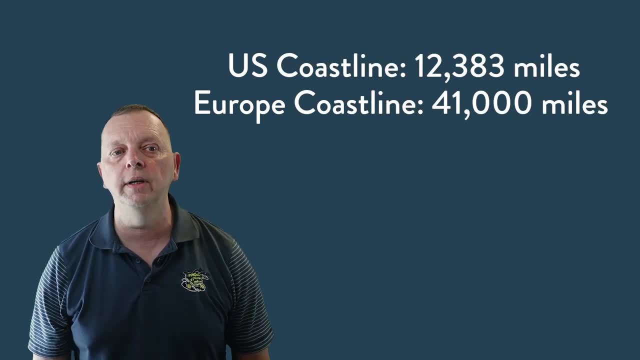 Now, despite the United States and Europe being in roughly the same land size, because Europe is a peninsula, a peninsula of peninsulas. remember, it has nearly three times the amount of coastline than that of the United States. This drives the importance of the seas to Europe. 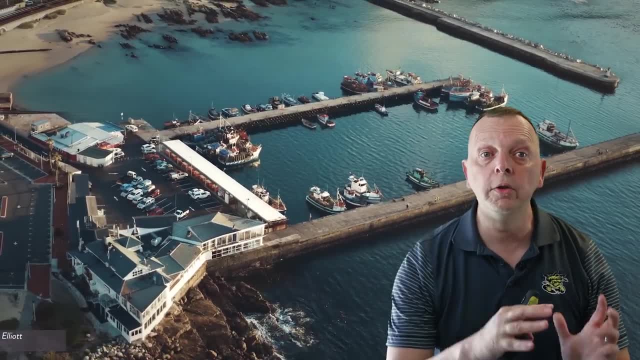 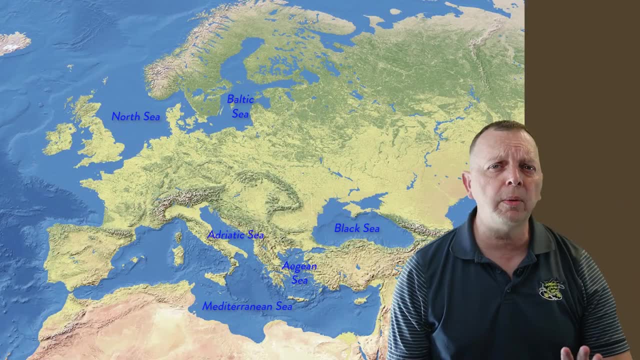 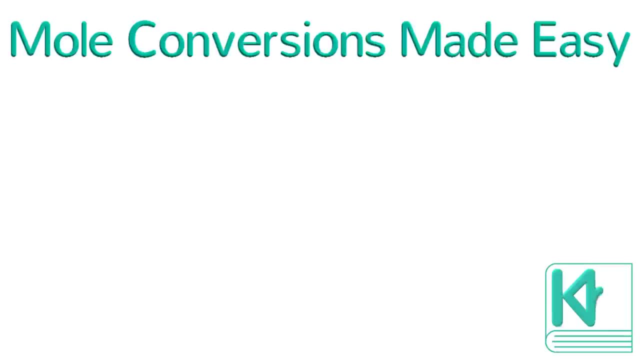 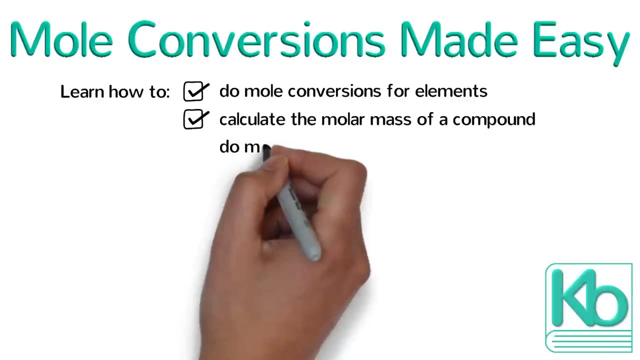 Welcome to Mole Conversions Made Easy, brought to you by Ketzbook. In this video, we're going to learn how to do mole conversions for elements, how to calculate the molar mass of a compound and how to do mole conversions for compounds. 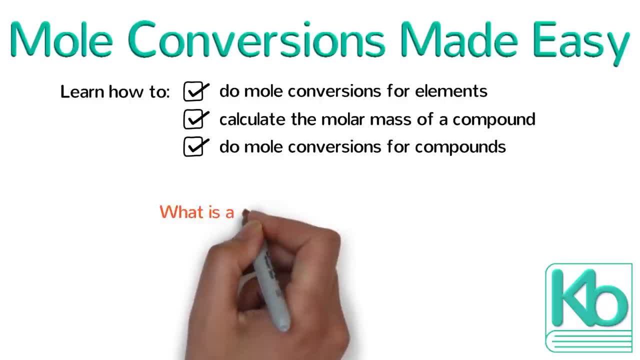 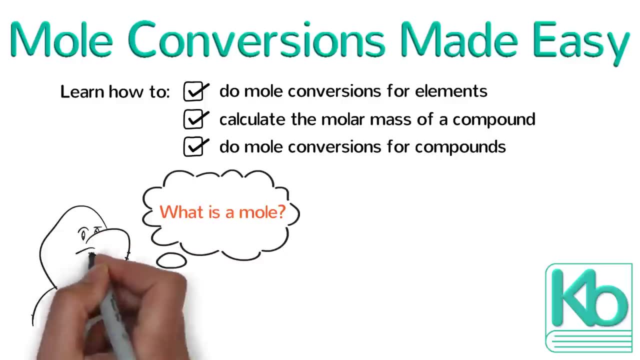 But before we jump into all that, you might be wondering: what is a mole? Well, there are lots of different moles in the world, but in chemistry a mole is simply a large number of things. It's kind of like a dozen, only bigger. 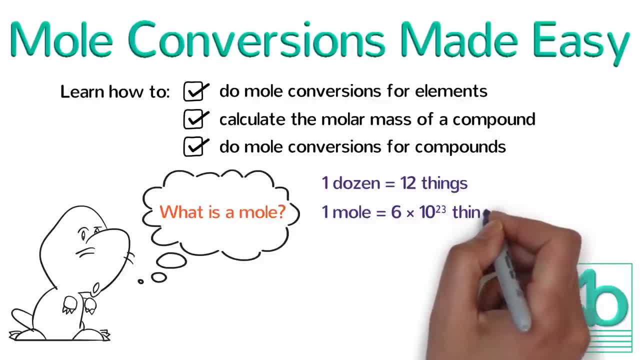 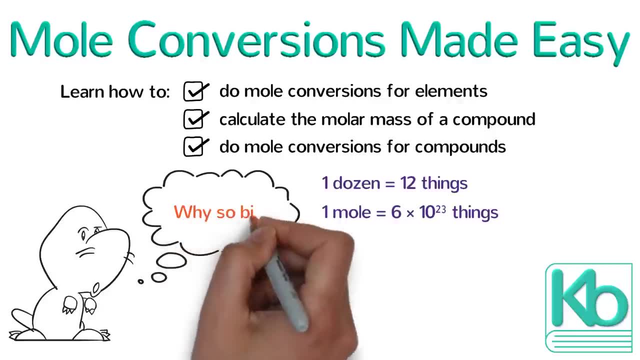 One dozen is 12 things. one mole is 6 times 10 to the 23rd things. That is 600 billion trillion things. Now, that's a lot of things. But why is the mole such a big number? Because atoms are so small. 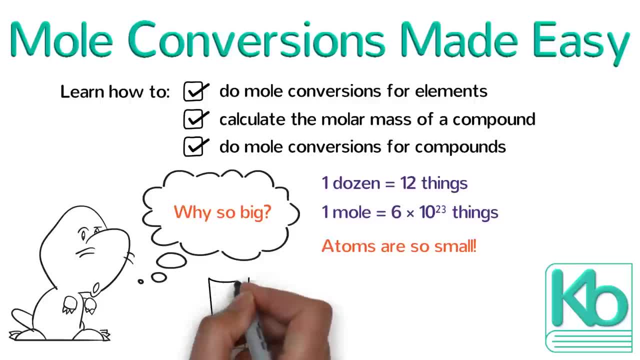 Suppose you wanted to know how many hydrogen atoms are in one cup of water. If you were able to count all the atoms, you would find that there are about 15 trillion trillion hydrogen atoms in a cup of water. But if we count using moles instead,